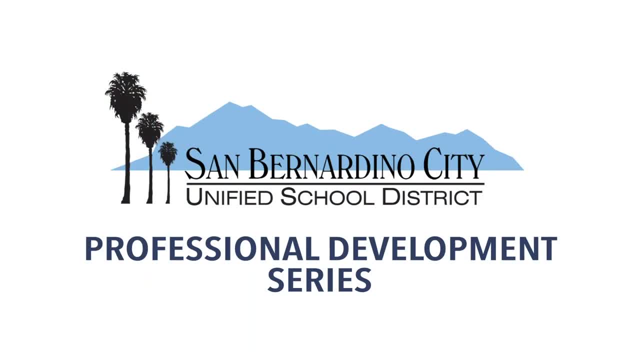 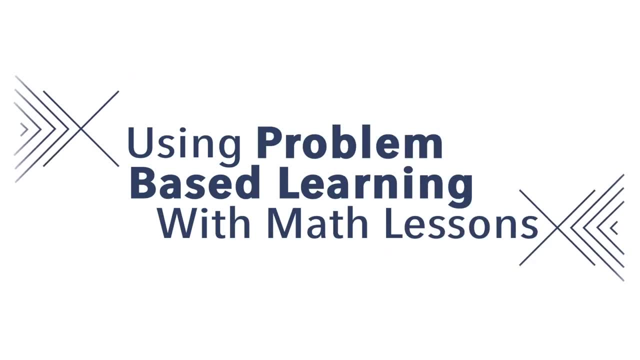 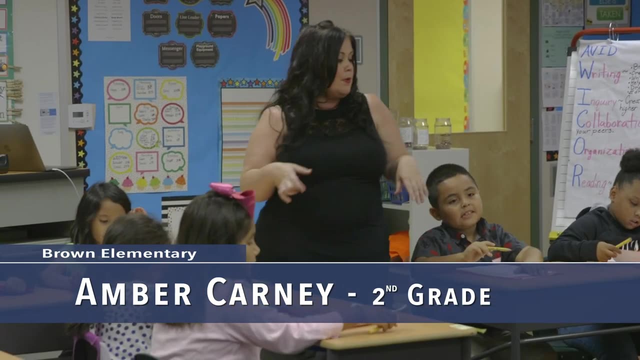 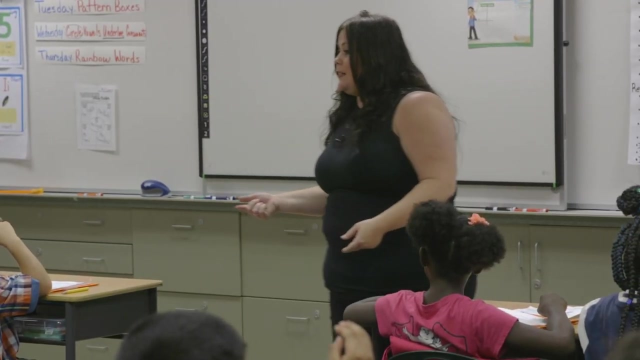 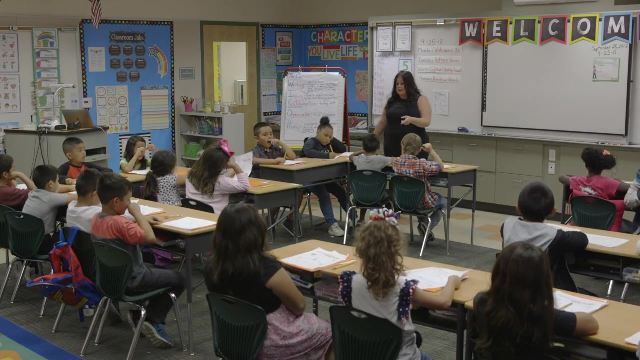 While you wait for me, look at the center box where you have your topic. Remember, I always leave off part of the title of the topic because you're trying to figure out the lesson through your problem. Good job, Jaden Through the problem. So look at that middle box. Make sure your PBL is in front of you. 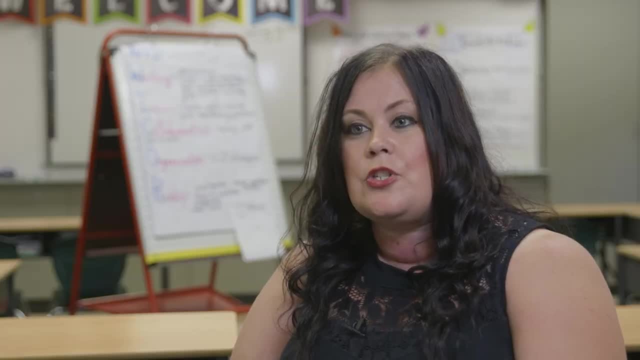 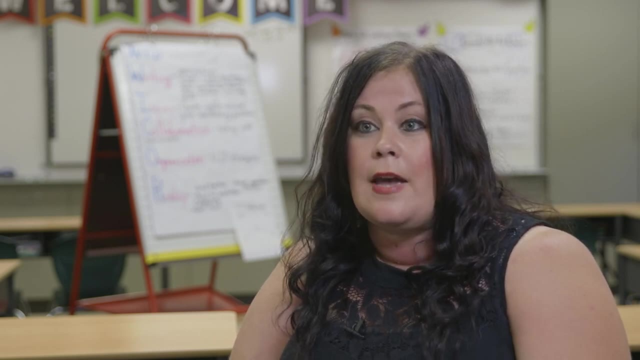 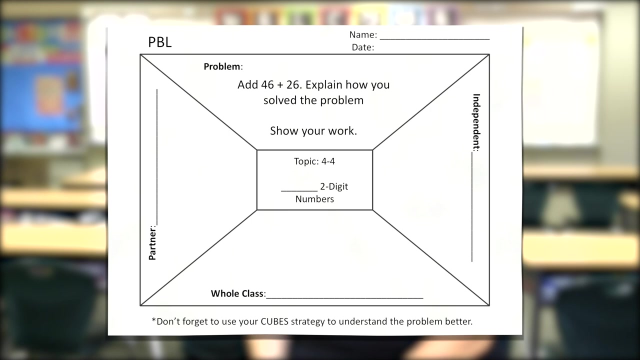 So problem-based learning is basically switching the teaching around, So you are no longer doing direct instruction where you are just teaching everything as a teacher. So for problem-based learning I developed a graphic organizer that looks a lot like the GATE template. It has the box in the center where I pose the topic. 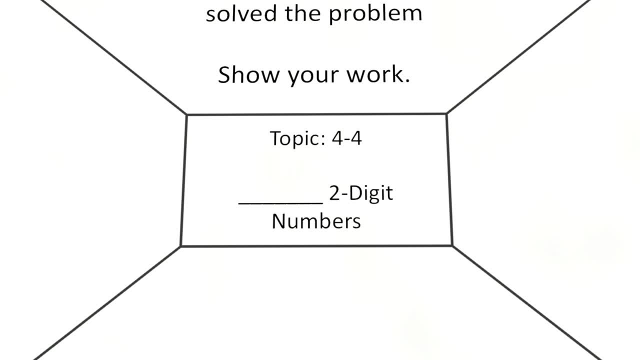 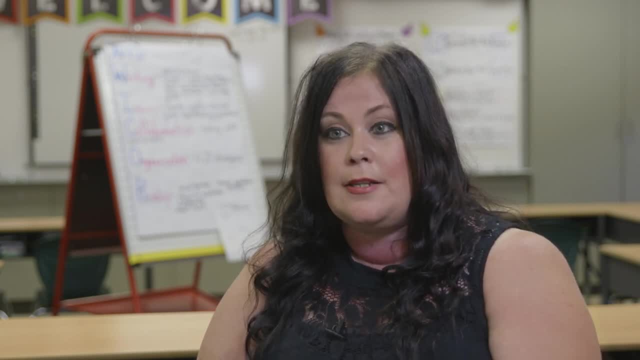 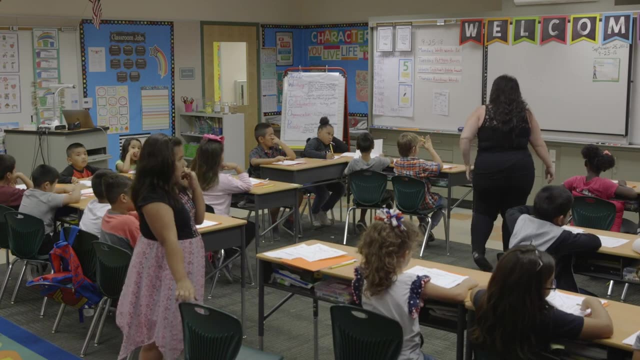 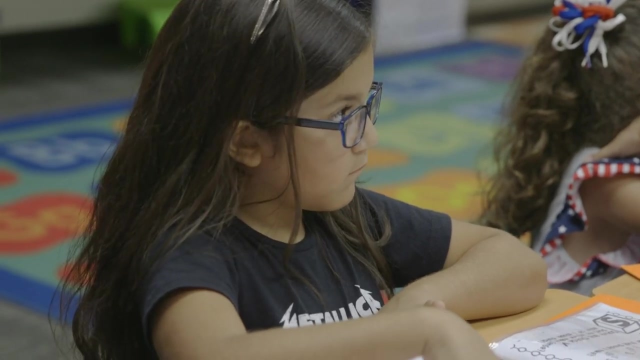 But then I only do part of the title, because oftentimes in the curriculum the title already is telling them what the lesson is going to be In problem-based learning. you want them to get there on their own? Okay, topic 4-4, blank. read the rest with me. Two-digit numbers. We're going to do something with two-digit numbers. 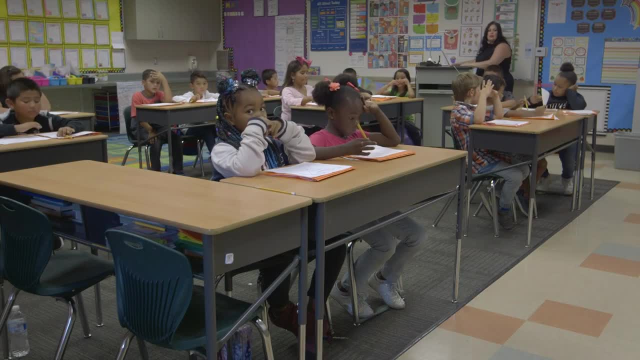 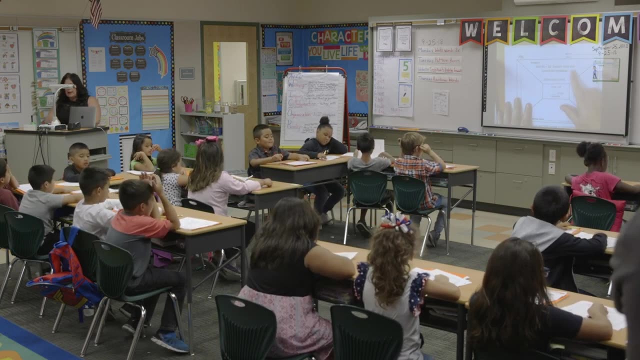 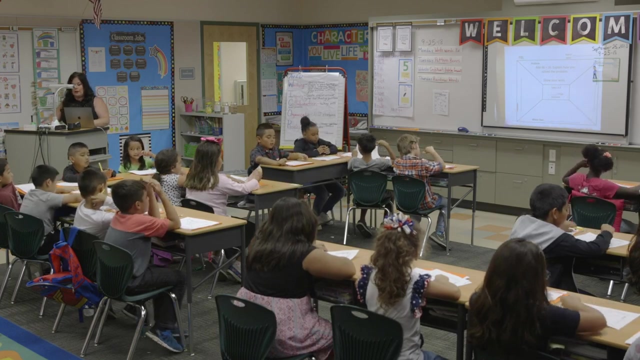 Okay, let's go to the problem box On your PBL sheet, Add 26.. Explain how you solved the problem And, last part, show your work. Very good, What do we use to better understand your problem? Raise your hand. 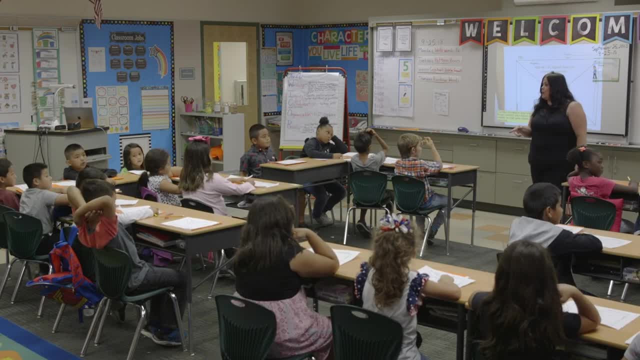 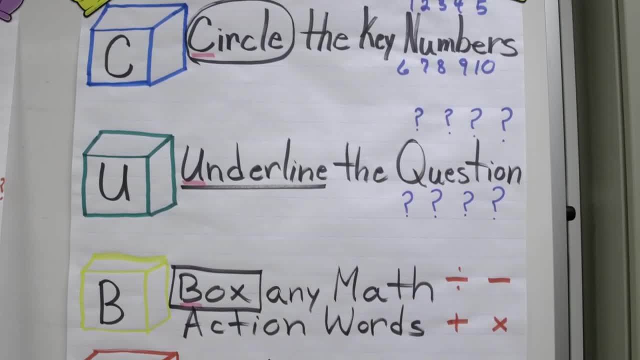 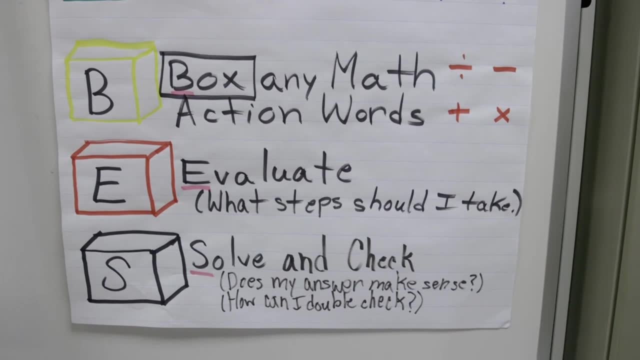 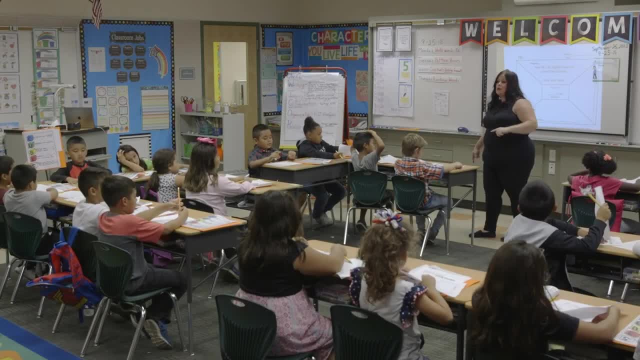 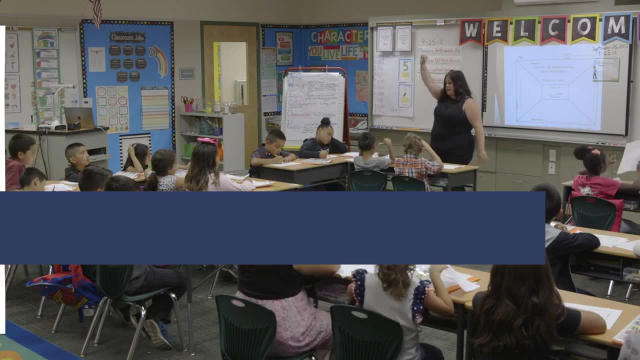 First we use CUBES, but they're four digits at the top. there We use number four, see two, three, eight and a half. All right, All right, Okay, Okay. so what do I want to do next? I need those our a really keep to just a to take a grip. 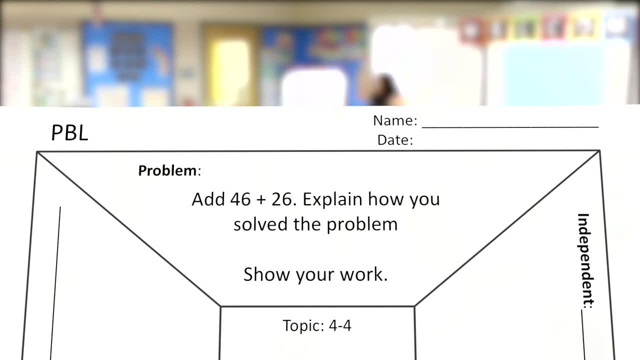 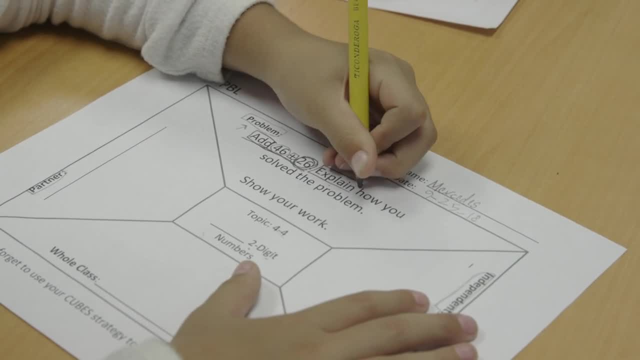 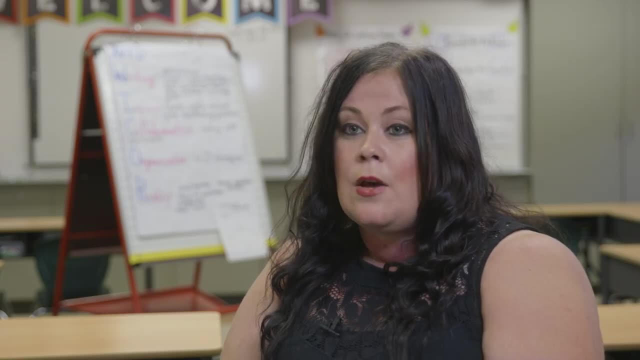 and that's where I have the problem typed and I have that there. so when we use the cube strategy, they are able to write on the problem. they're doing all the steps. they're circling boxing. you're able to see their annotations. so after we break up the problem with cubes, we move to the independent box, where now 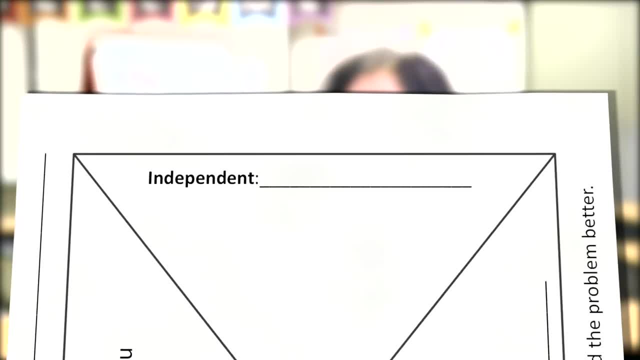 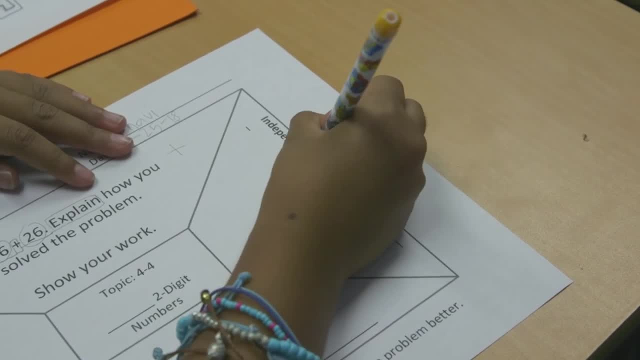 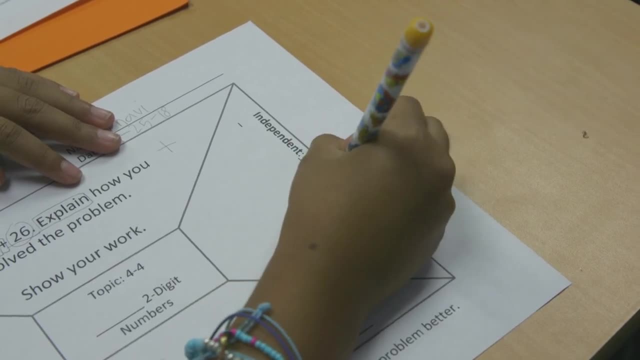 the students have an idea of what operation or how or how they're going to solve the problem. think about your strategy. write what you're gonna use. so you're not solving yet, you're just writing your strategy on top. the first step is just you getting your minds going, because the real work is gonna be. 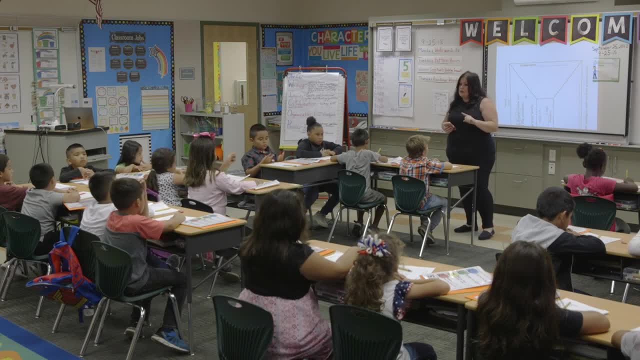 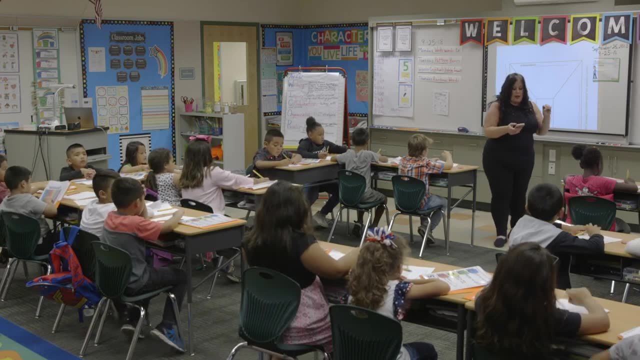 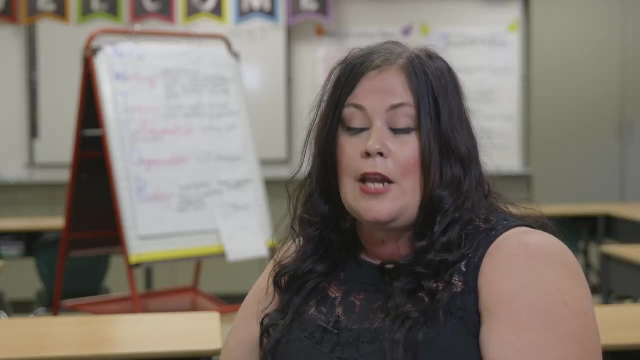 when you talk to your partner, right? so I'm gonna let you work for two minutes by yourself. independent is voice level zero. two minutes to solve this problem. go in this step as the teacher. I'm not expecting them to get it right. I mean, I would hope that they would, but for me, my expectancy is for them to get their. 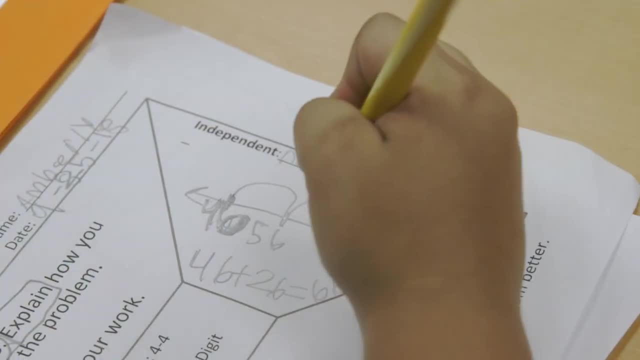 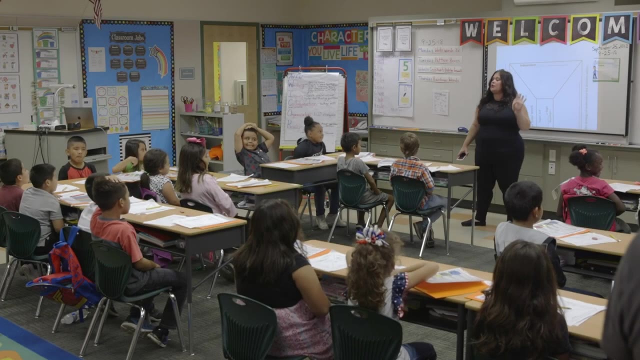 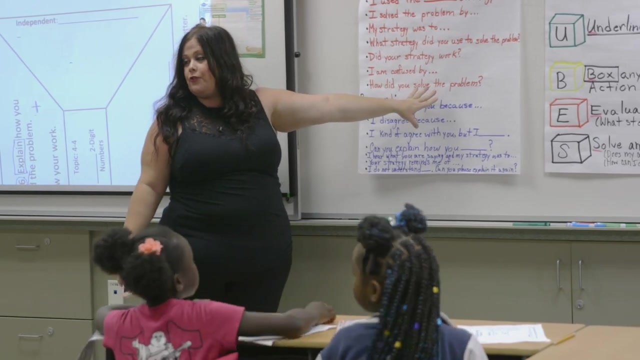 mind going to be able to choose a strategy and to be able to explain why they chose that. so you're gonna keep looking and you're independent because now when you talk to your partner and you have that discussion piece, using your math talk sentence frames, you're explaining. 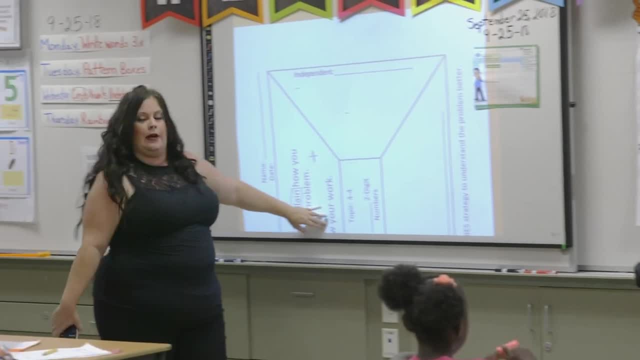 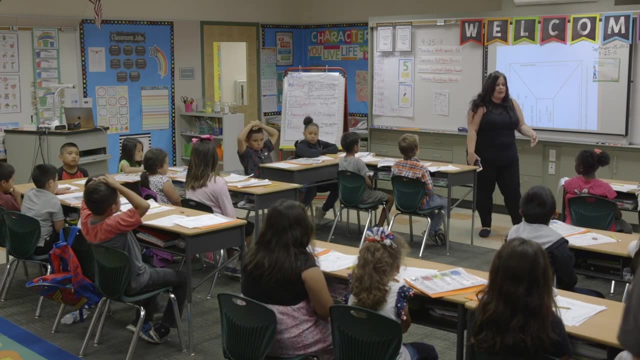 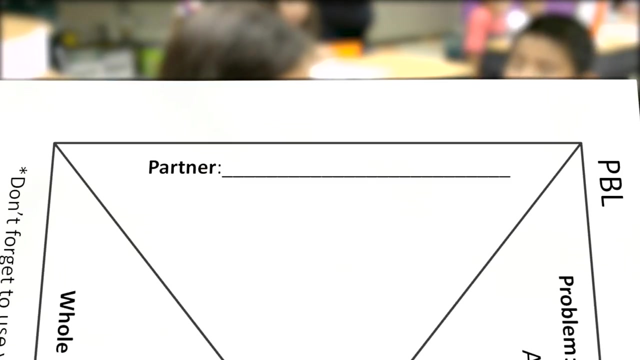 your work. you're doing the show your work part. you show your. you should have showed it. so now, not only gonna tell your partner what you used, what strategy, but explain it in the partner box. they first discussed with their partner using their math talk sentence frames what they did. 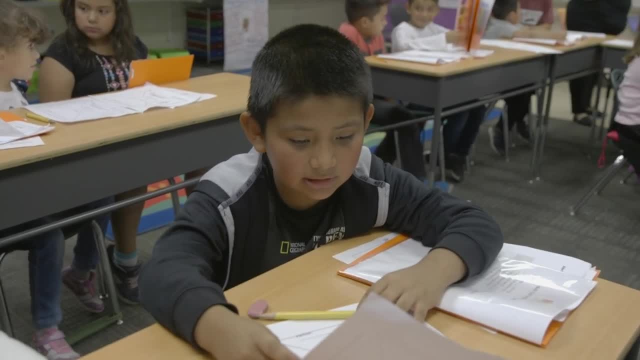 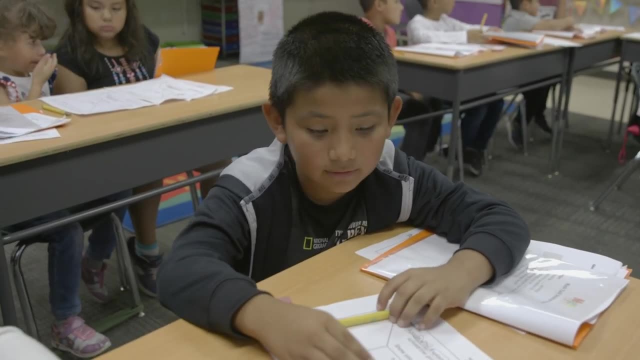 I use cubes because it's an easy strategy to use by putting your mind to it. i use cubes because it's an easy strategy to use by putting your mind to it. Make sure you responded. Eventually we'll lead into where they're discussing and solving on their own. 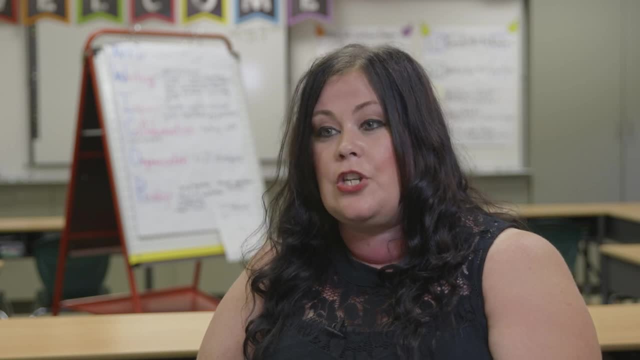 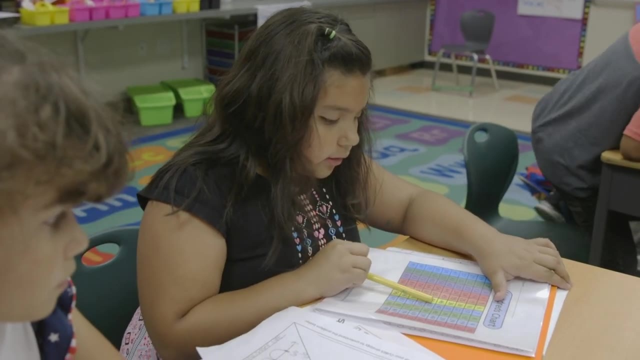 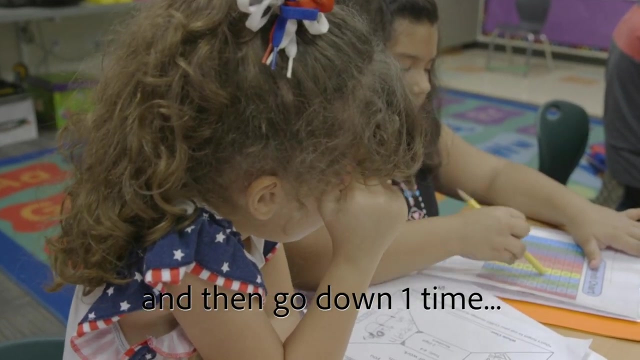 So I set the timer. let them talk for about a minute and decide within each other what strategy they want to use if they want to keep theirs. but they have to pick one together, 46. And then go down one time. 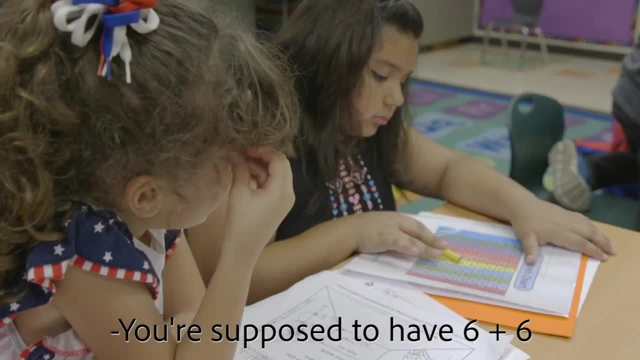 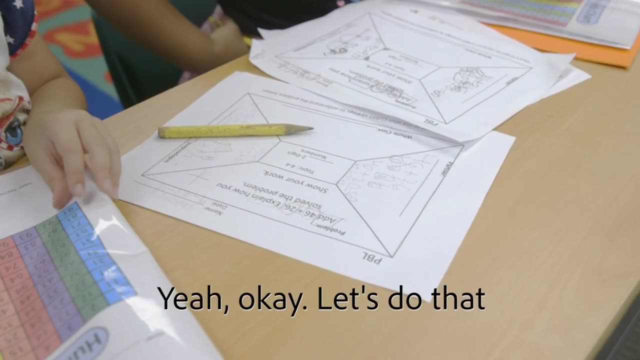 Wait, 6.. Oh Wait, what 6 plus 6.. 6 plus 6.. Yeah, OK, Let's do that One more minute. What is 6 plus 6? 12. 12. OK, 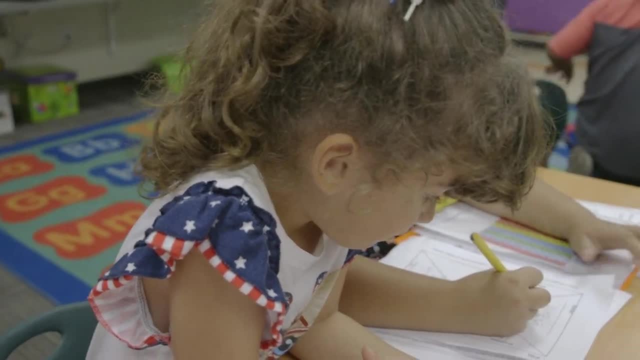 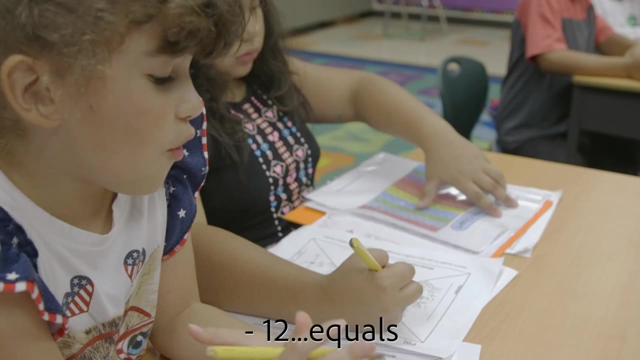 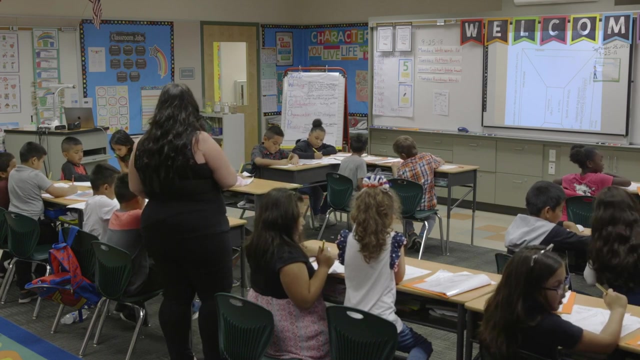 So we're going to add a parking lot, 12. 12. OK, That equals 12.. You know that During that time, during the partner time, I'm watching, I'm walking around And I'm picking those students who are going to help lead the class to that lesson. 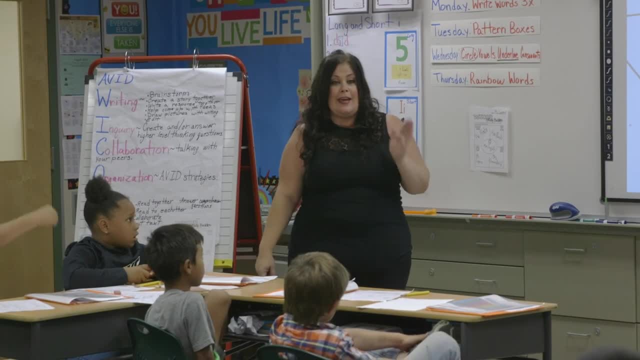 So they're going to be the models, They're going to be the teachers. So, Mercedes and Aiden, you want to show us your strategy. Last one, And this is going to lead to our lesson: We're going to do more of this today. 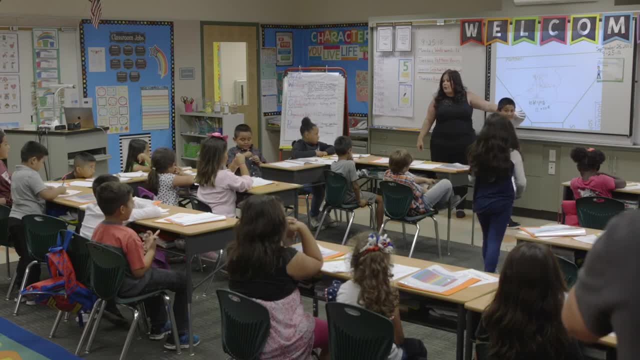 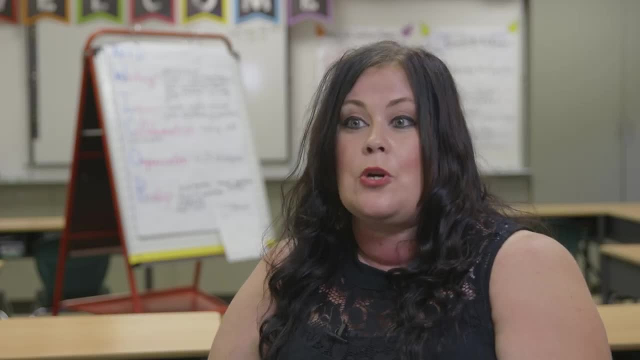 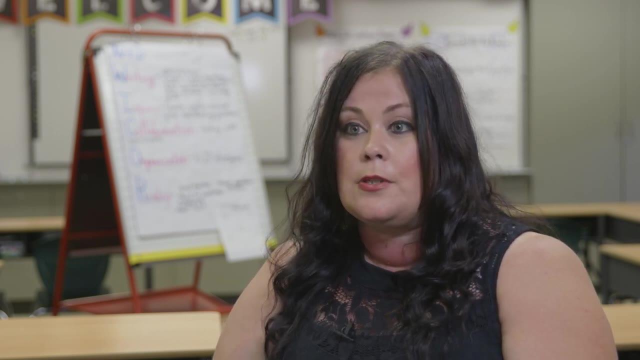 And it goes with the place value. blocks Ready? OK, Let's give them our attention. So now they think it's time for them to show off their answers, Whereas, again, you, as the teacher, know where the lesson's going. So now you have chosen two to three groups who come up and explain. 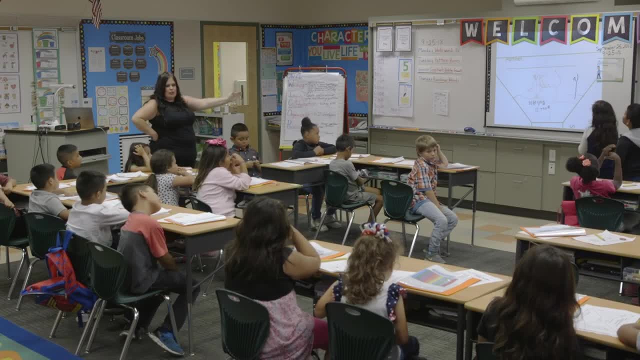 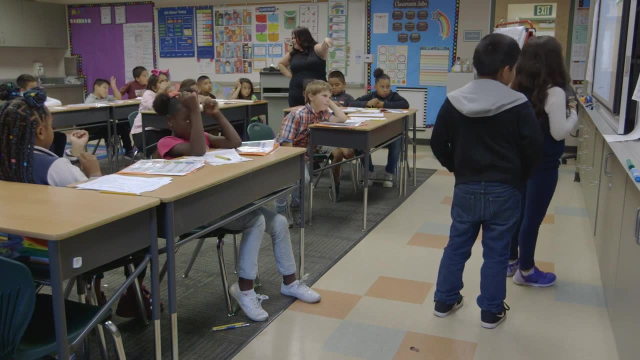 And the whole class is listening, So this should look familiar. She just did a chart. She just said you're splitting it into what Mercedes Tens and 1. What does this look like? 5. 5. Our math problem we used today, right? 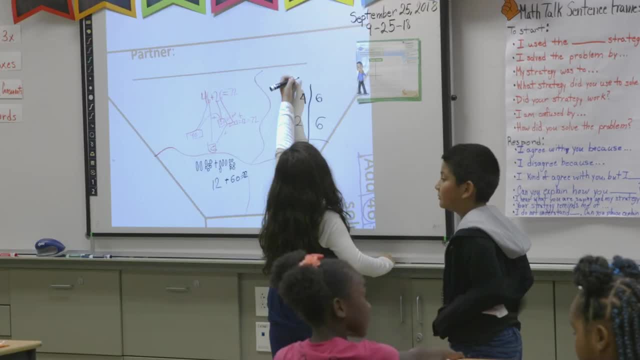 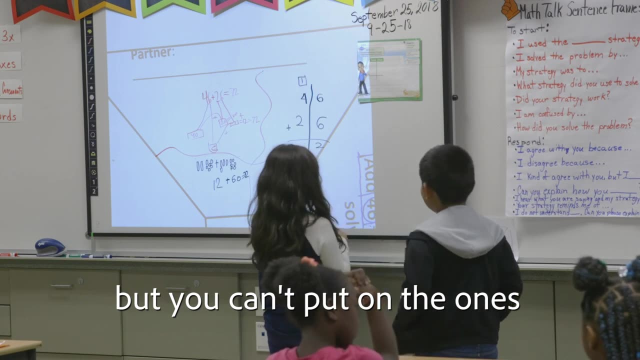 So you split up your 1s and your 10s. Now I'm going to be quiet. It's hard for me. So, Mercedes and Aiden, Go ahead, Jump in Go. This is specifically for 12.. But you can't put on the 1s, because the 1 is a 10.. 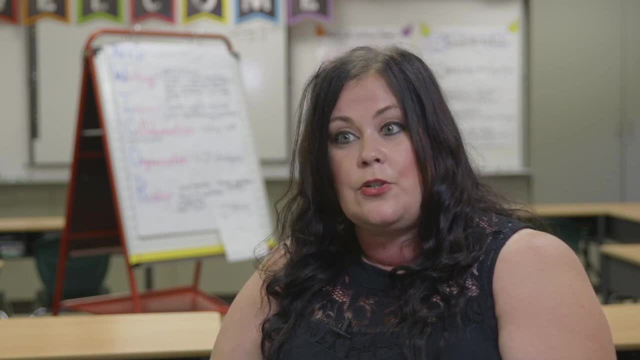 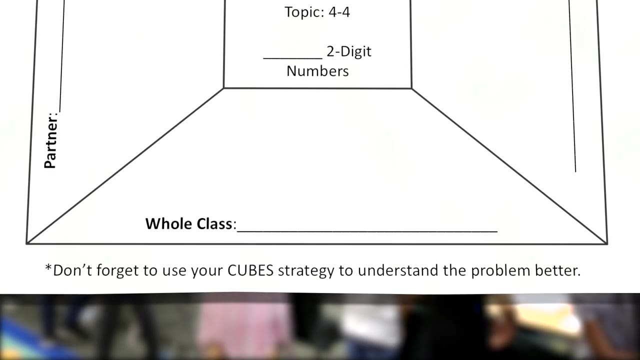 And then, once you get the students up there and they lead the direction you want, that's the strategy you choose to do as a whole class. You are now, you're taking over as the teacher, But they still don't know that The students are thinking that they're still leading it. 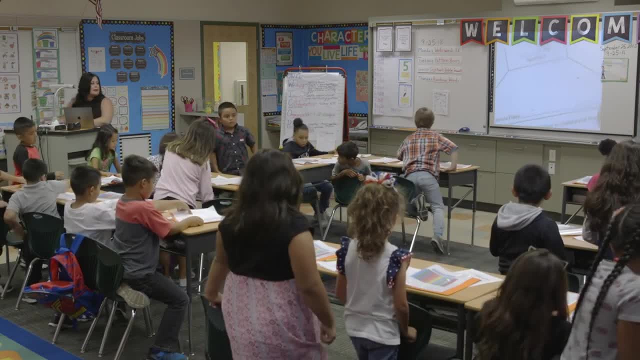 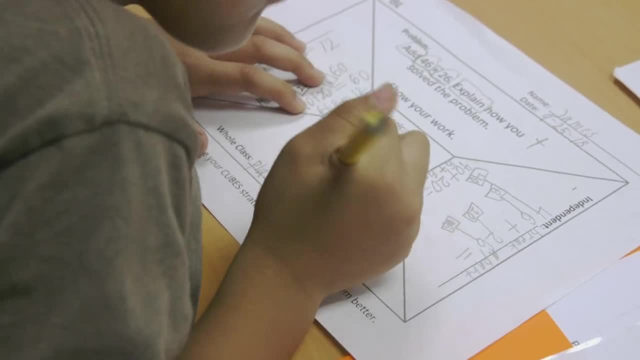 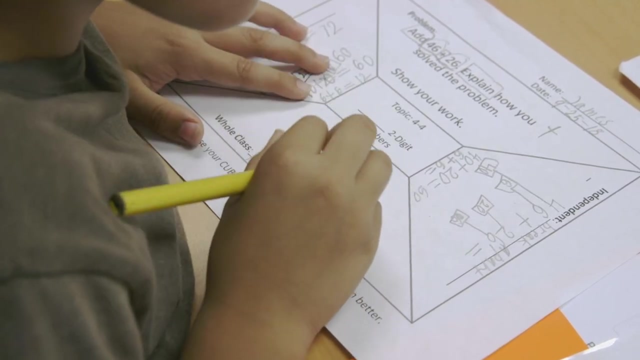 Turn to the your paper, to the whole class, And we're going to use two strategies. We're going to use the place value blocks to model And then we're going to add using place value with regrouping. Let's draw each group first.